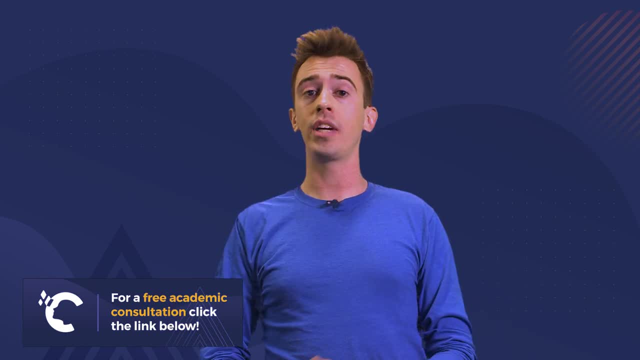 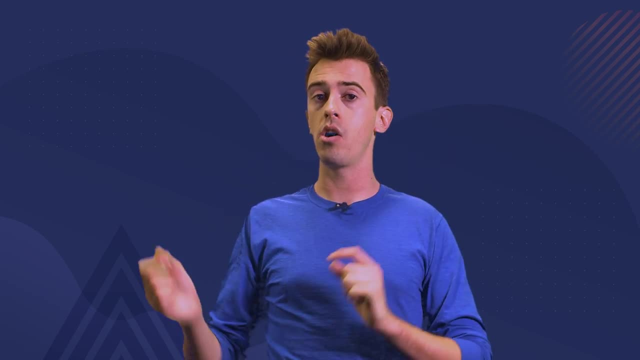 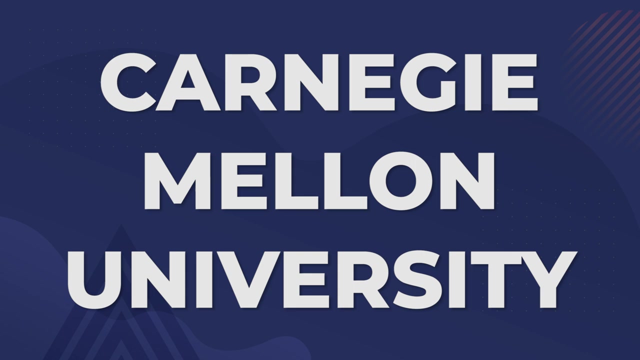 want to study. please click the link below and you'll get connected up with one of our academic experts on a free consultation to send you on to the school of your dreams. So let's get started. Number 10 on our list is Carnegie Mellon University, or CMU, located in Pittsburgh. The Statistics and 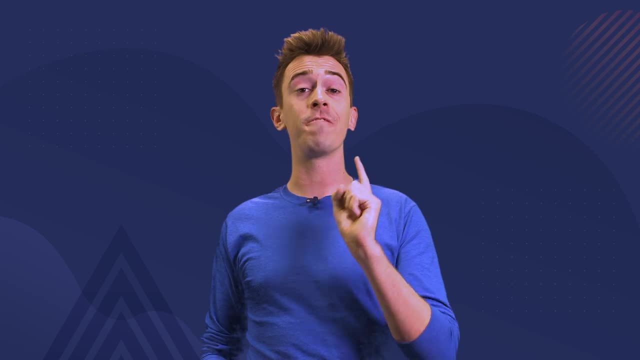 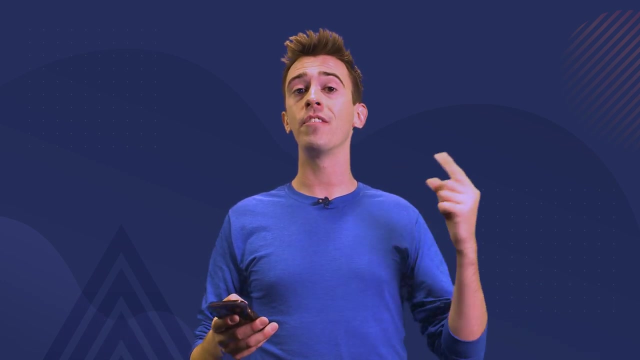 Data Science program at CMU places a large emphasis on flexibility, allowing its students to apply their statistics to a particular field, such as math or statistics learning, to a number of real world problems. You can focus on a number of different tracks at CMU, including stat, core, stat, machine learning, economic. 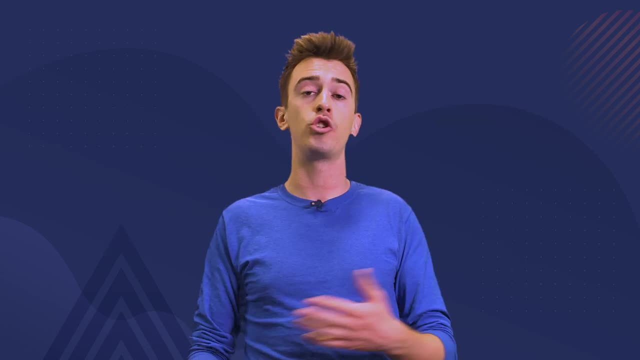 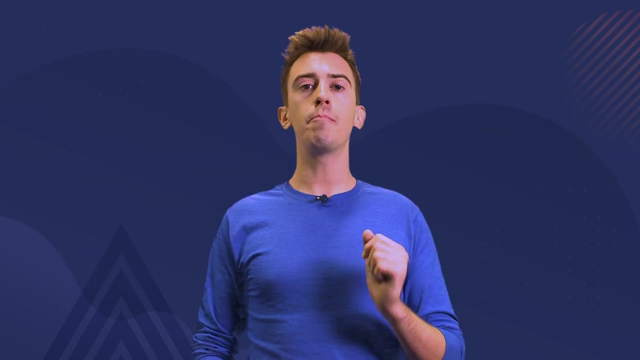 stats, math stats and neuro stats, all of which can be applied to a wide range of disciplines. Number 9 on our list is the National University of Singapore, or NUS. The Department of Statistics and Applied Probability at NUS offers two distinct 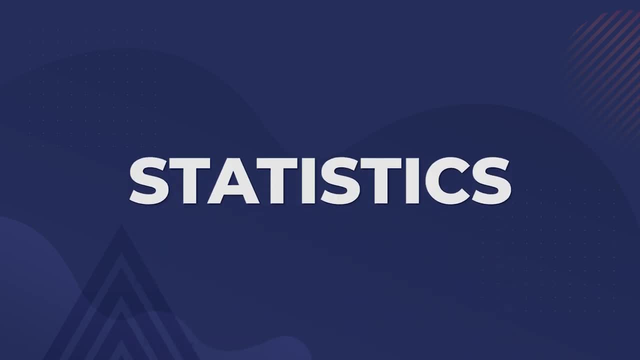 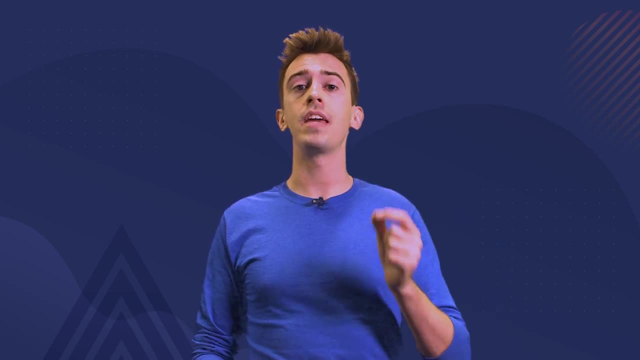 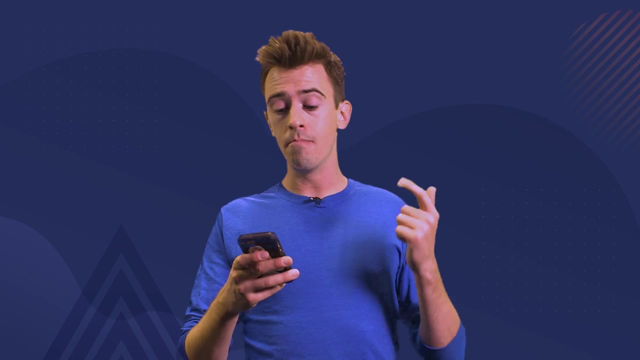 degrees within statistics. The first is just statistics and the second is data science and analytics. NUS offers several applied research concentrations within their statistics and data science departments. The focus of those includes quality control and engineering, marketing, research, finance, economics. 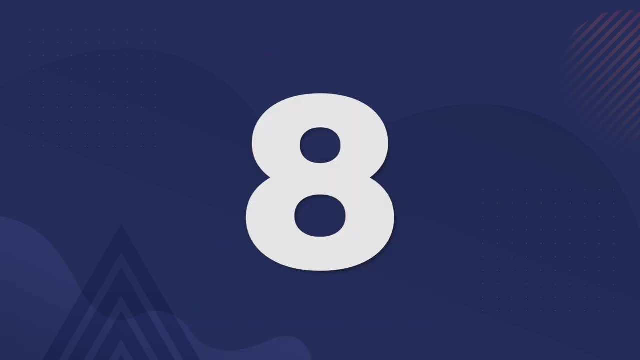 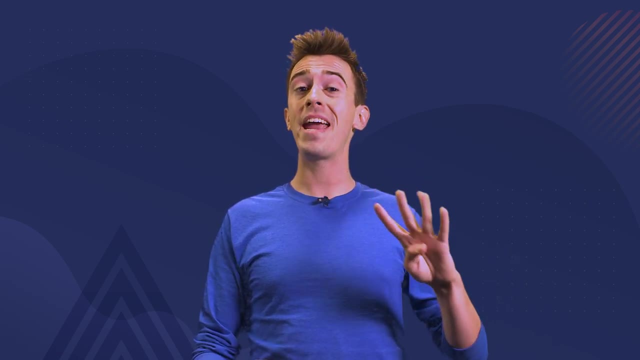 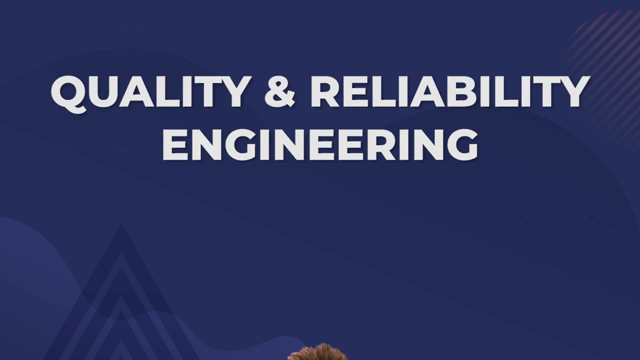 survey methodology and statistical genetics. Number eight on our list is the Georgia Institute of Technology. Statistics research at the Georgia Institute of Technology focuses on four main application areas, which are advanced manufacturing, logistics, health informatics and digital technology, And quality and reliability engineering. And if you're a student at the Georgia Institute of Technology. you'll also probably do a lot of work with other outside research organizations, including Children's Healthcare of Atlanta, the Chinese Academy of Sciences in Beijing and the Centers for Disease Control and Prevention. Number seven on our list is University of Oxford's Department of. Statistics At Oxford, you can either get a three-year BA program or a four-year master's program with a focus on mathematics and statistics, which is a collaboration with their world-renowned mathematics department Research specialties in the Department of Statistics at the University of Oxford. 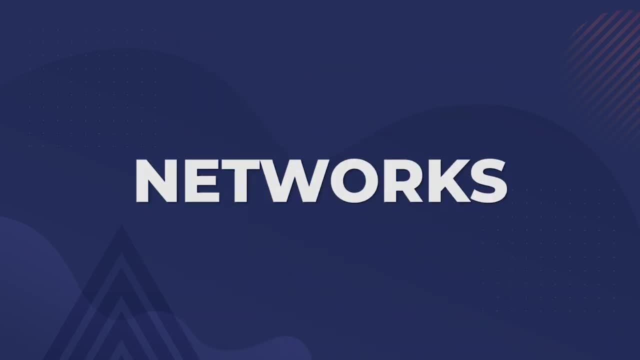 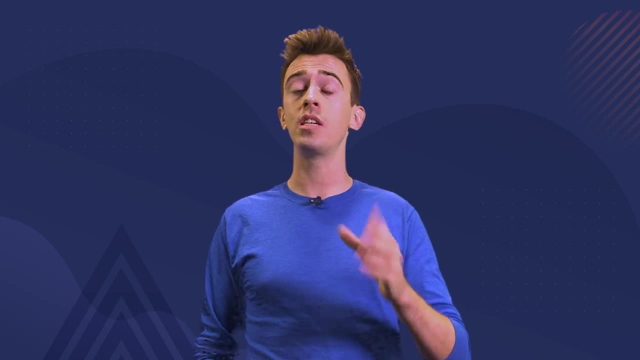 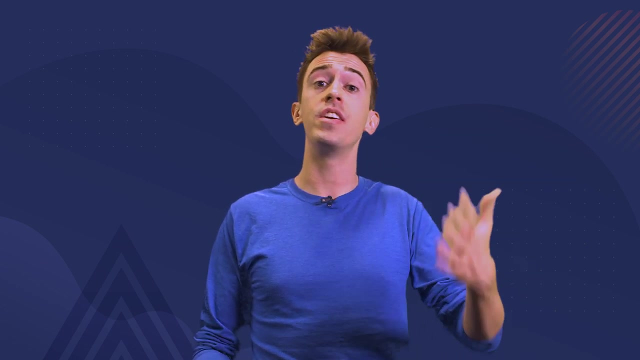 include machine learning, genomics and networks. Number six on our list is the University of California, Berkeley. The statistics program at UC Berkeley prides itself on not only pushing students to focus on methodology and on the theory behind statistics, but also on applying a lot of that research and a lot of that. 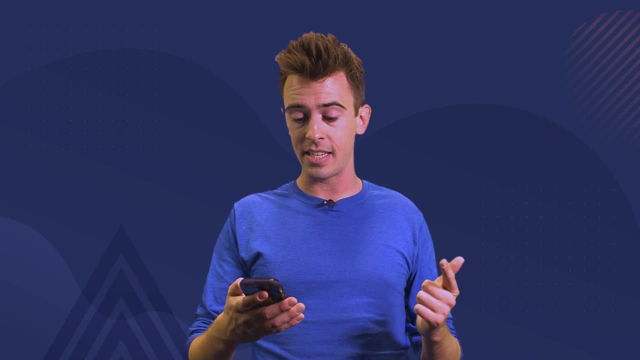 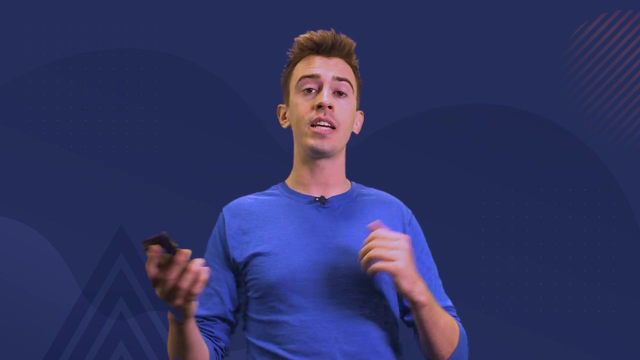 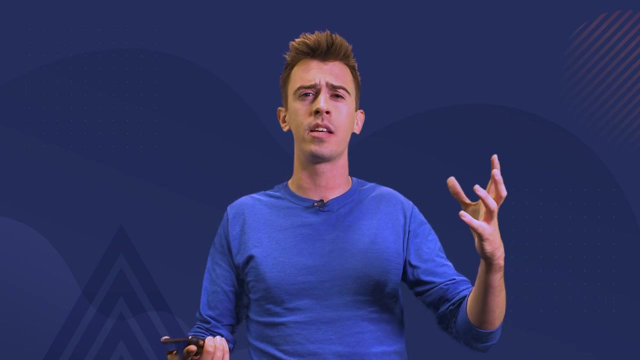 work to real-world problems such as AIDS research, the US Census and neurophysiology. Berkeley is also home to the Berkeley Statistics Industry Alliance program, which connects students and faculty with many industry leaders really across industries. It creates this. 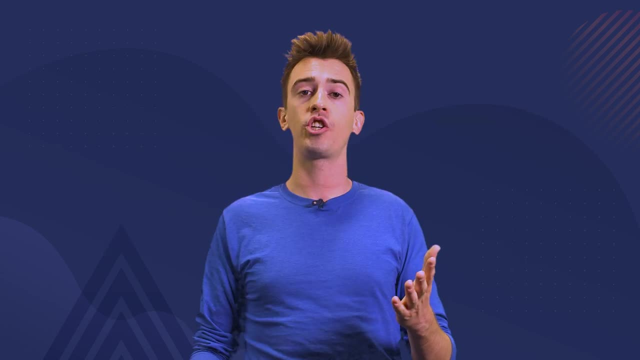 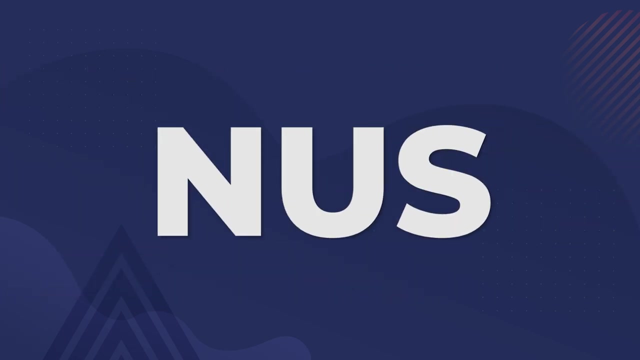 problems. You can focus on a number of different tracks at CMU, including stat, core stat, machine learning, economic stats, math stats and neuro stats, all of which can be applied to a wide range of disciplines. Number nine on our list is: 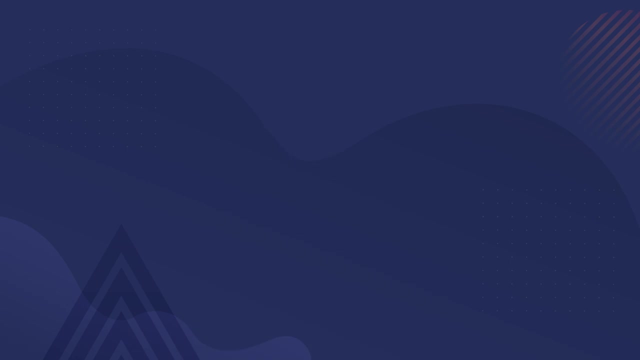 the National University of Singapore, or NUS. The Department of Statistics and Applied Probability at NUS offers two distinct degrees within statistics. The first is just statistics and the second is data science and analytics. The Department of Statistics and Applied Probability at NUS offers two distinct degrees within statistics. The first is just statistics and the second is data science and analytics. 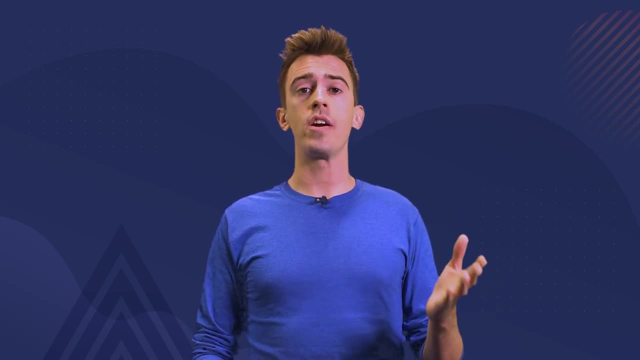 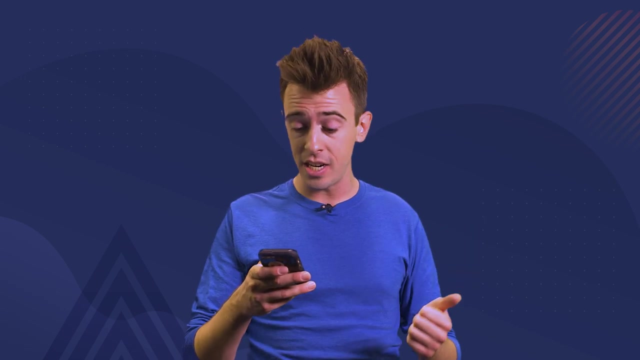 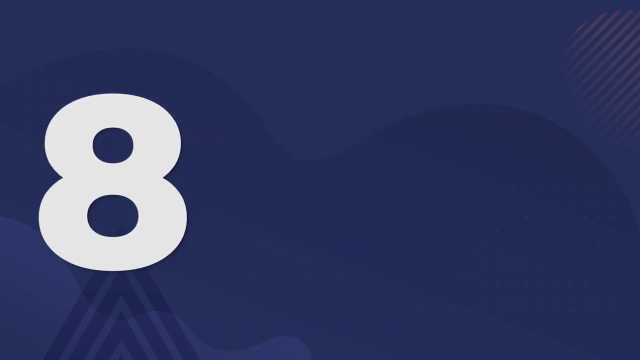 NUS offers several applied research concentrations within their statistics and data science departments. The focus of those includes quality control and engineering, marketing research, finance, economics, survey methodology and statistical genetics. Number eight on our list is the Georgia Institute of Technology. 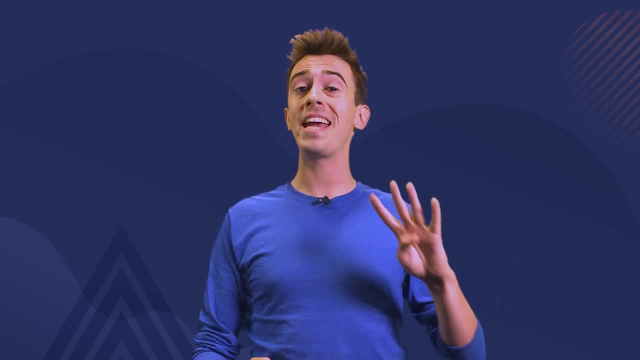 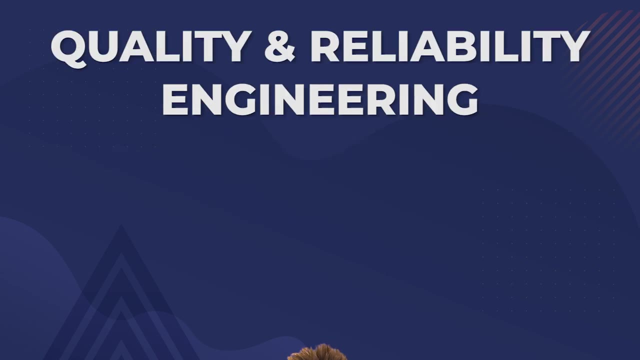 Statistics research at the Georgia Institute of Technology focuses on four main application areas, which are advanced manufacturing, logistics, health, informatics and quality and reliability engineering. And if you're a student at the Georgia Institute of Technology, you'll also probably do a lot. of work with other outside research organizations, including Children's Healthcare of Atlanta, the Chinese Academy of Sciences in Beijing and the Centers for Disease Control and Prevention. Number seven on our list is University of Oxford's Department of Statistics. At Oxford, you can either get a three-year BA program. 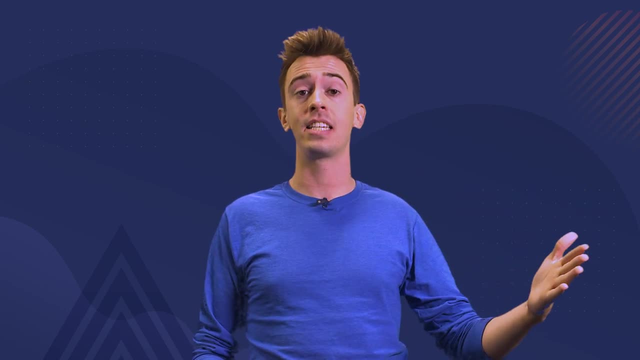 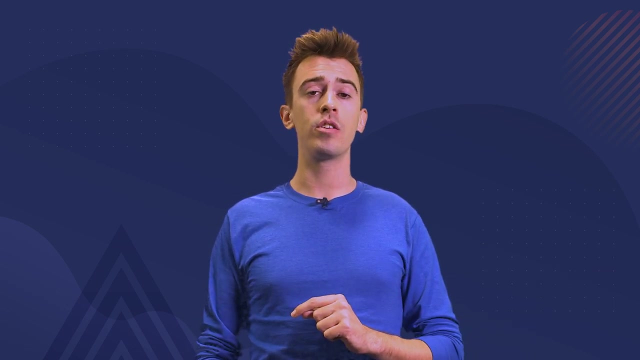 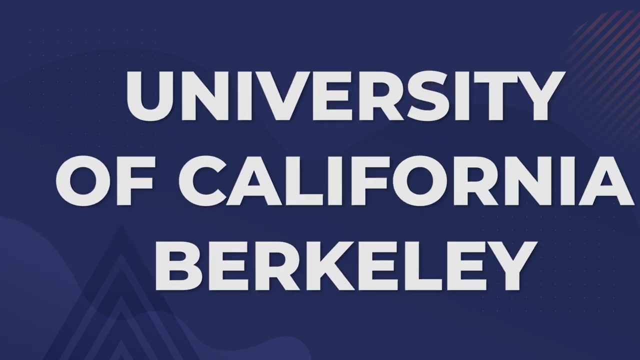 Or a four-year master's program with a focus on mathematics and statistics, which is a collaboration with their world-renowned mathematics department. Research specialties in the Department of Statistics at the University of Oxford include machine learning, genomics and networks. Number six on our list is the University of California, Berkeley. 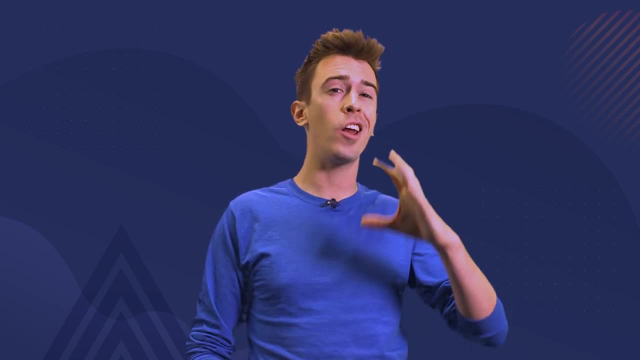 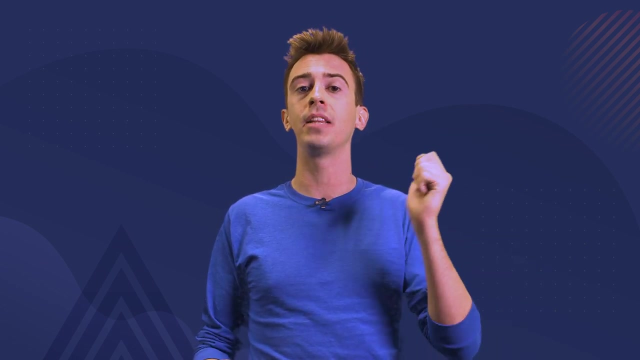 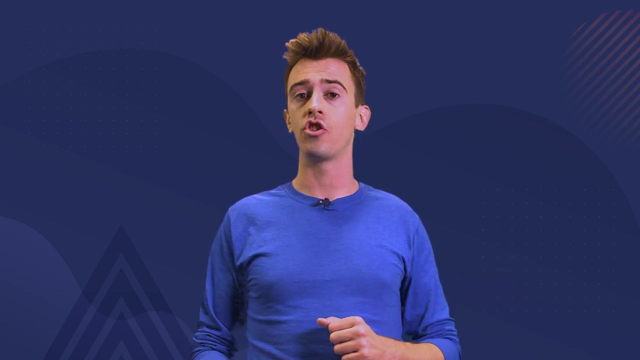 The statistics program at UC Berkeley prides itself on not only pushing students to focus on methodology and on the theory behind statistics, But also on applying a lot of that research and a lot of that work to real-world problems such as AIDS research, the US Census and neurophysiology. 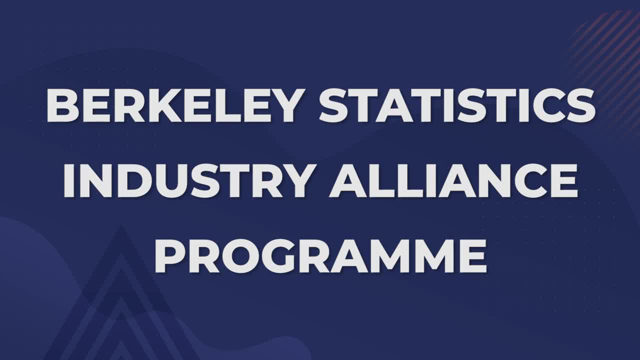 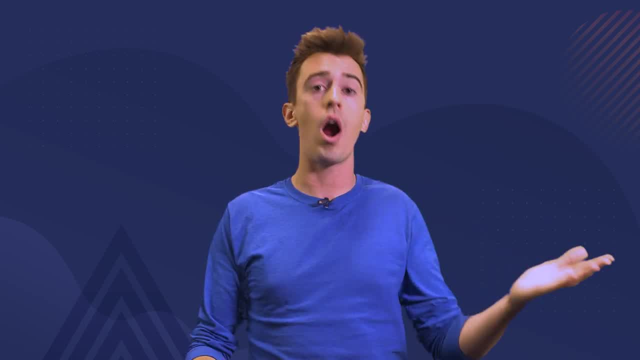 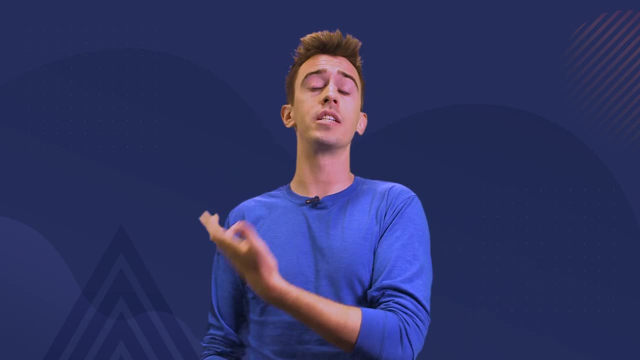 Berkeley is also home to the Berkeley Statistics Industry Alliance program, which connects students and faculty with many industry leaders, really across industries. It creates this very cool sort of connection between the private sector and UC Berkeley's faculty and research. Number five on our list is the University of Cambridge and their Department. 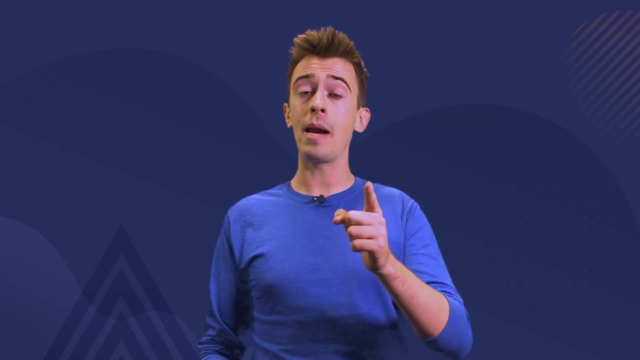 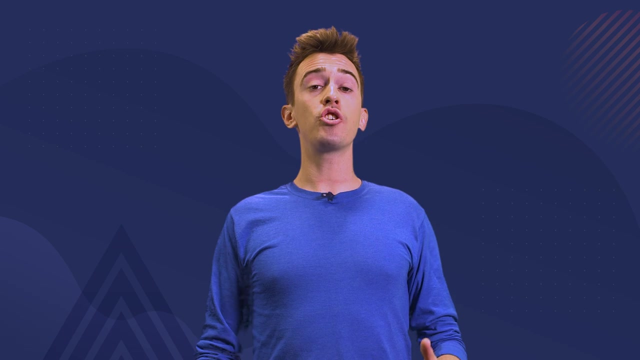 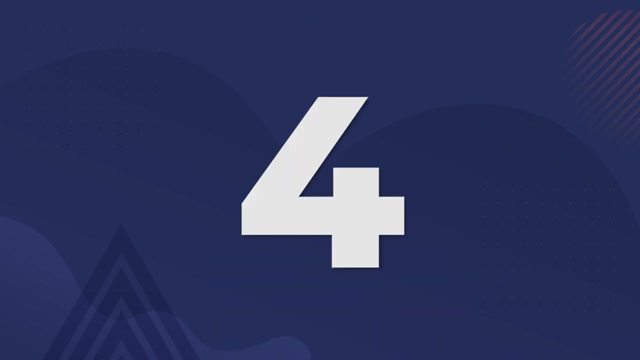 of Mathematics and Mathematical Statistics. University of Cambridge faculty has also won six Fields Medals. That's great. Cambridge is home to the Statistics Clinic, which offers free statistical consulting services to all university members, regardless of what department they're in. Number four on our list is ETH Zurich. 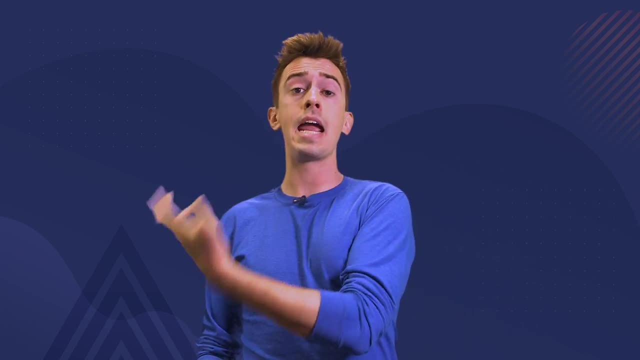 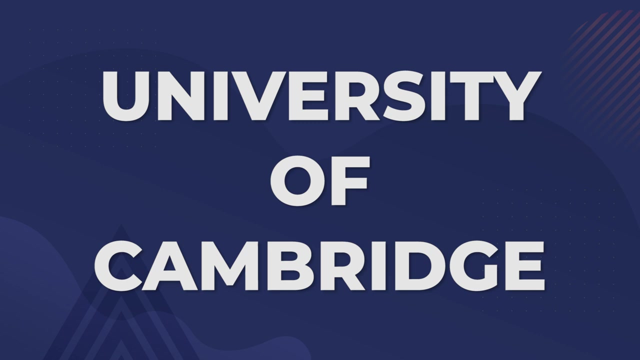 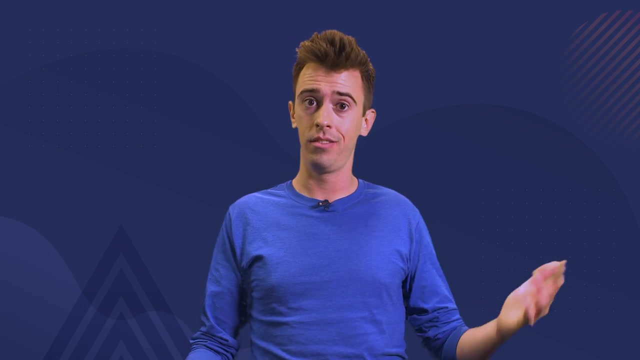 very cool sort of connection between the private sector and UC Berkeley's faculty and research. Number five on our list is the University of Cambridge and their Department of Pure Mathematics and Mathematical Statistics. University of Cambridge also won six Fields medals. That's great. Cambridge is home to the 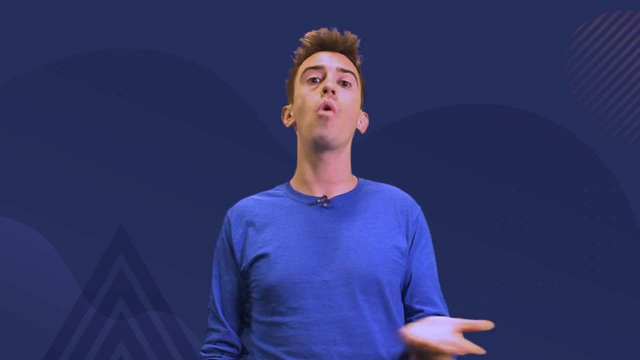 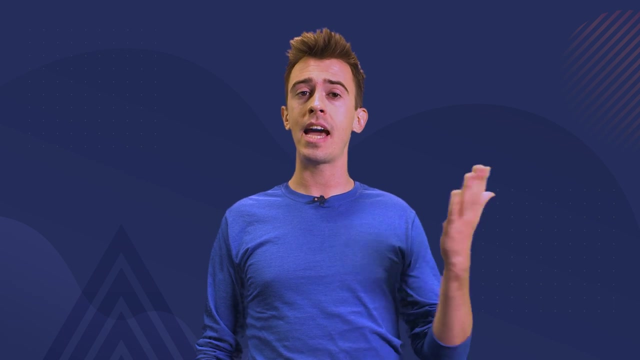 Statistics Clinic, which offers free statistical consulting services to all university members, regardless of what department they're in. Number four on our list is ETH Zurich. If you're studying statistics at ETH Zurich, you're probably studying it in the Department of Mathematics or in the Department of 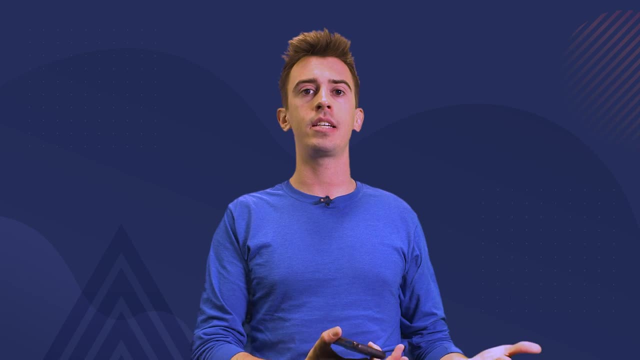 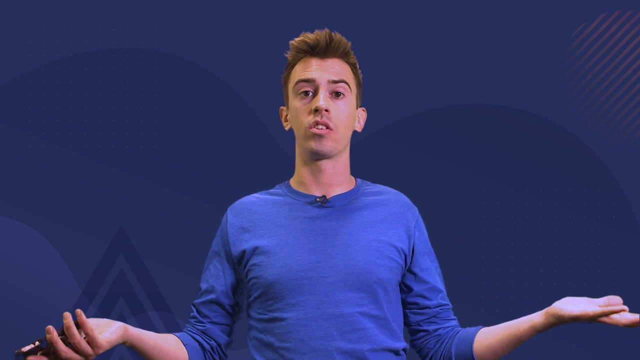 Computational Science and Engineering. Both of these departments approach statistics and approach the research in slightly different ways, of course, but in any case you're getting one of the best statistical programs in the world. Number three on our list is Stanford University. You can't major in statistics. 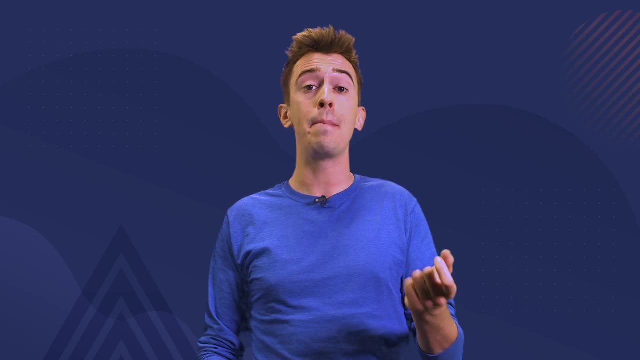 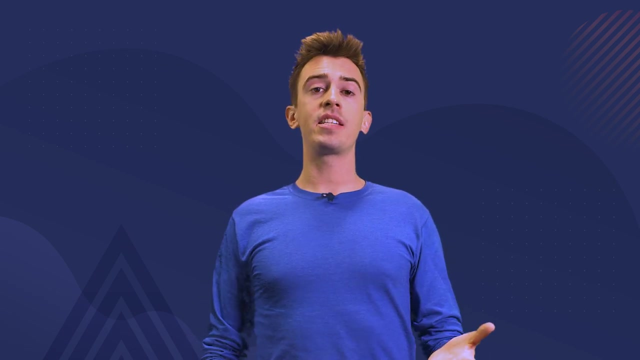 at Stanford, but they encourage students who are interested in statistics in majoring in Mathematical and Computational Science. However, you can get a statistics minor and a data science minor. Stanford prides itself on giving its students many opportunities to do statistical research during the 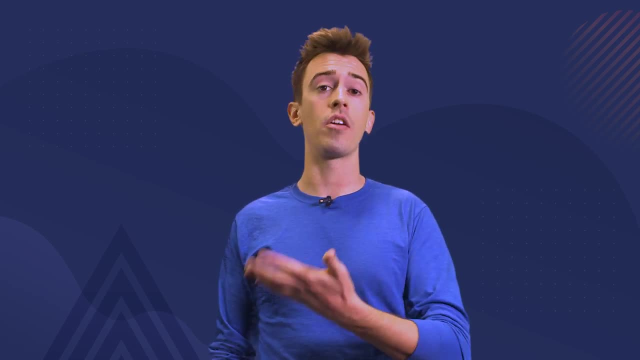 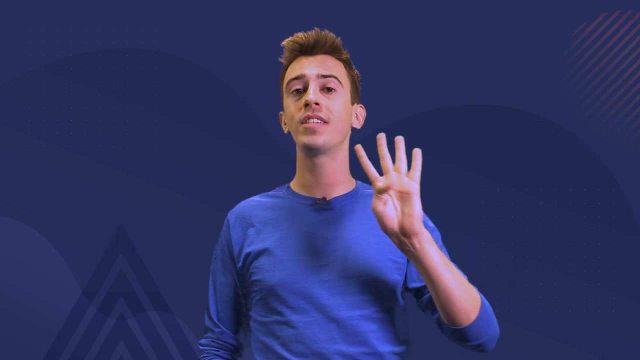 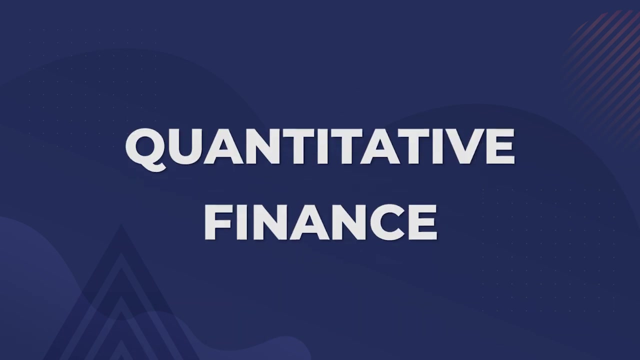 summer, oftentimes in collaboration with biology and other departments. Number two on our list is Harvard. Harvard Statistics offers four distinct tracks, and those are: one, core statistical principles and methods, two, data science, three, quantitative finance and four, bioinformatics and computational biology. If you study statistics at Harvard, you can probably go on to a lot of high-paying jobs at tech giants such as Google, at finance giants such as Goldman Sachs and at many other giants across industries. Statistics students at Harvard get a lot of money. 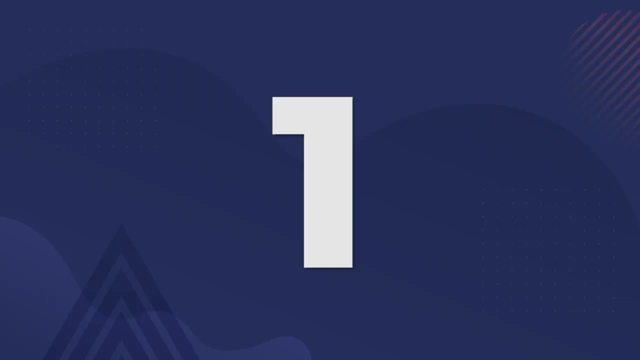 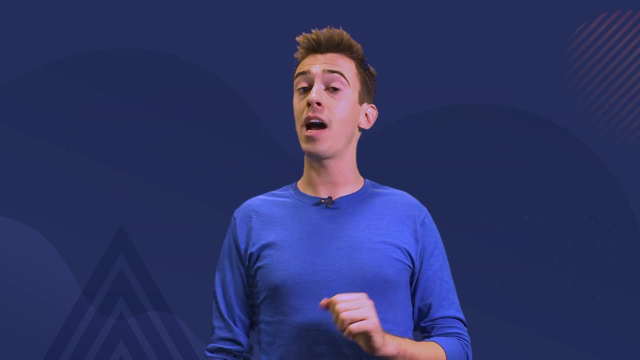 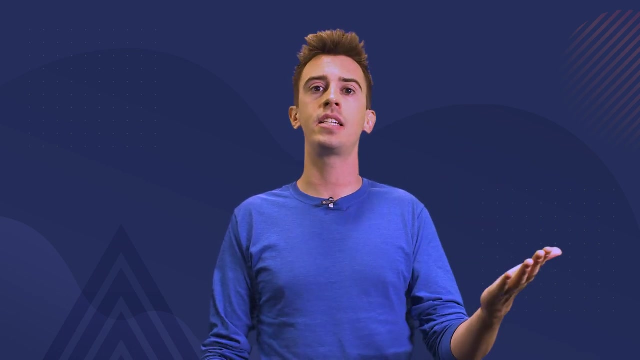 after they graduate. And the number one school on our list- no surprise to anyone- is the Massachusetts Institute of Technology. Now, MIT does not actually have a statistics department, but it is still the number one school on our list because they study statistics in many, many other departments. 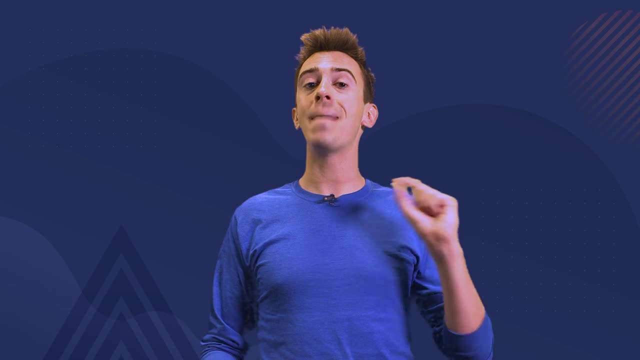 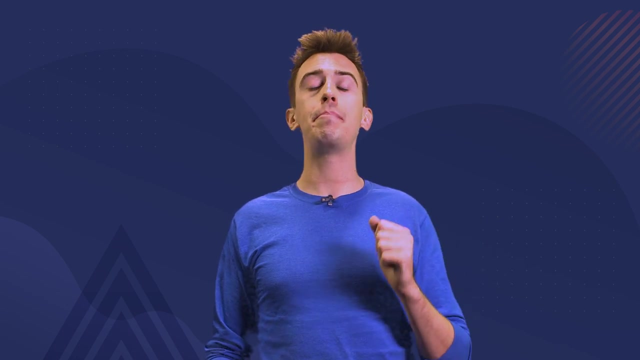 and they're the best in the world at doing it. You can, however, get a minor in statistics and data science at MIT, which is a pretty recent development, And after the undergraduate level, there is an interdisciplinary PhD in statistics that MIT offers, which much like its undergrad programs. 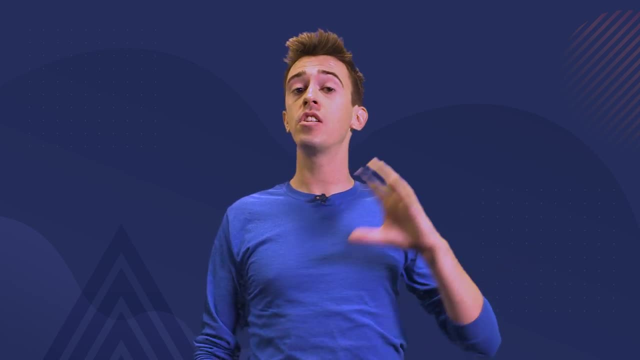 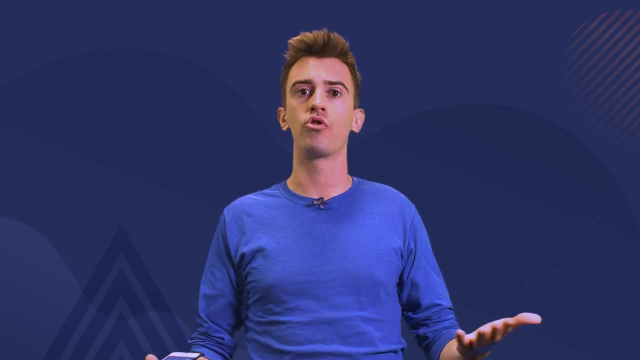 If you're studying statistics at ETH Zurich, you're probably studying it in the Department of Mathematics or in the Department of Computational Science and Engineering. Both of these departments approach the field of mathematics and statistics. They approach statistics and approach their research in slightly different ways, of course. 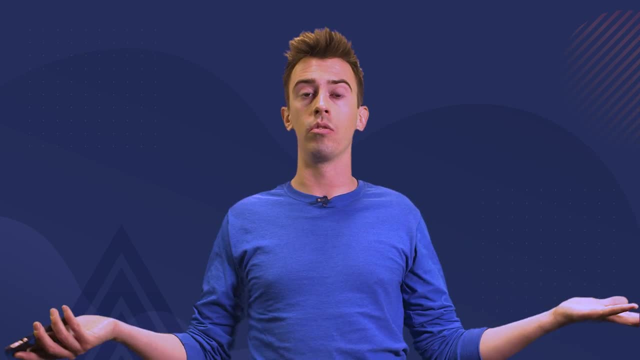 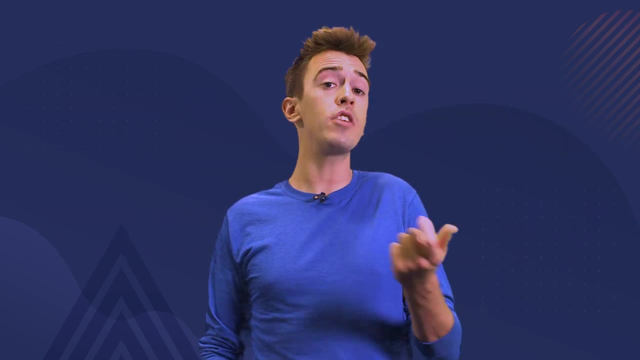 But in either case you're getting one of the best statistical programs in the world. Number three on our list is Stanford University. You can't major in statistics at Stanford, but they encourage students who are interested in statistics in majoring in mathematical and computational science. 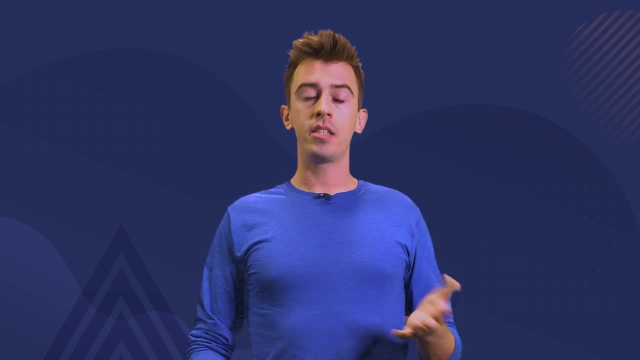 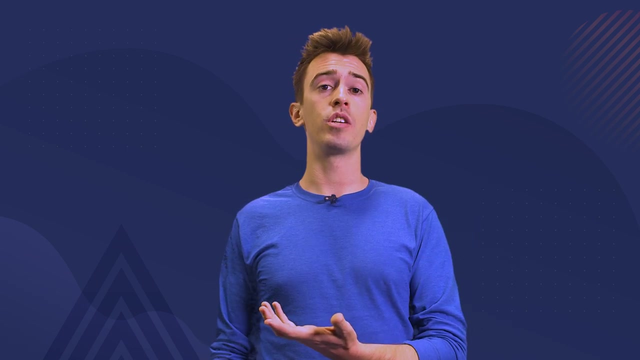 However, you can get a statistics minor and a data science minor. Stanford prides itself on giving its students many opportunities to do statistical research during the summer, Oftentimes in collaboration with the University of Cambridge. It's nothing new. Instead, the department prepares the students for work抧il climate and is aikid with 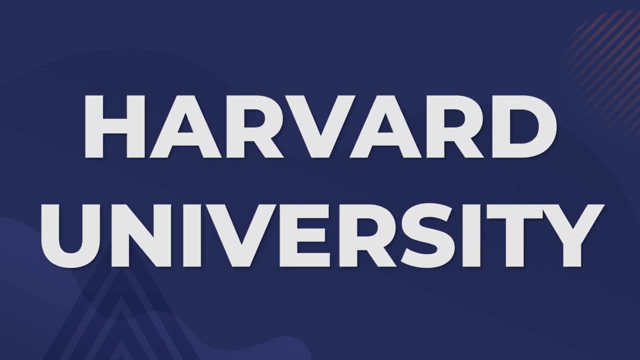 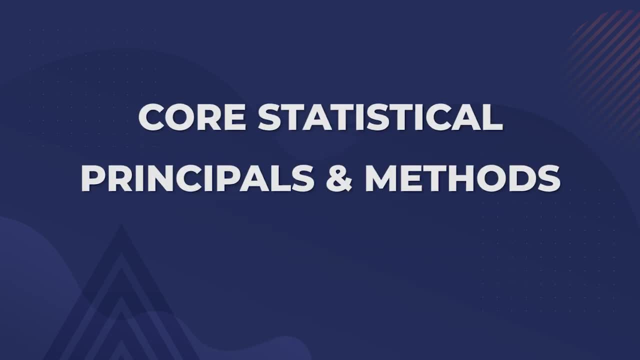 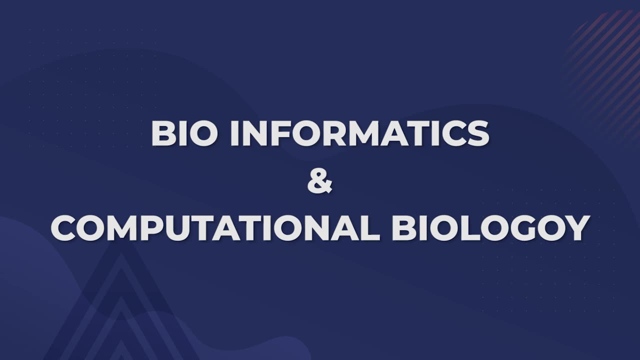 their skills. Number three on our list is Harvard University. Harvard Statistics offers four distinct tracks. Those are one, core statistical principles and methods, Two, data science. Three, quantitative finance and four, bioinformatics and computational biology. If you study statistics at Harvard, you can probably go on to a lot of high paying jobs. 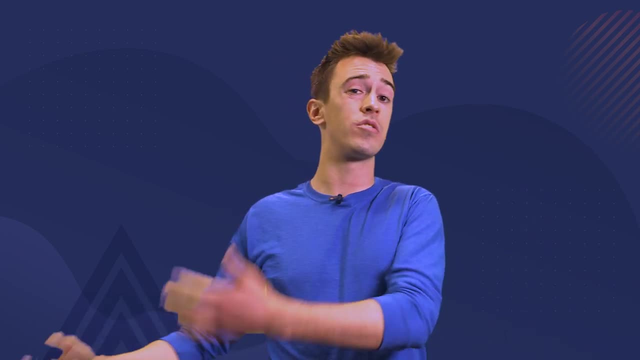 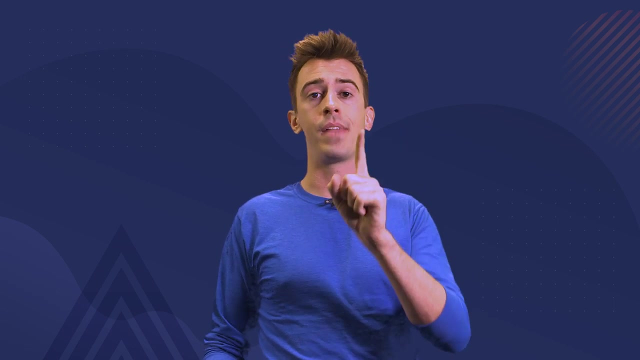 at tech giants such as Google, at finance giants such as Stanford or at other companies, And to be sure to subscribe to my YouTube channel. Have a great day as Goldman Sachs and many other giants across industries. Statistics students at Harvard get a lot of money. 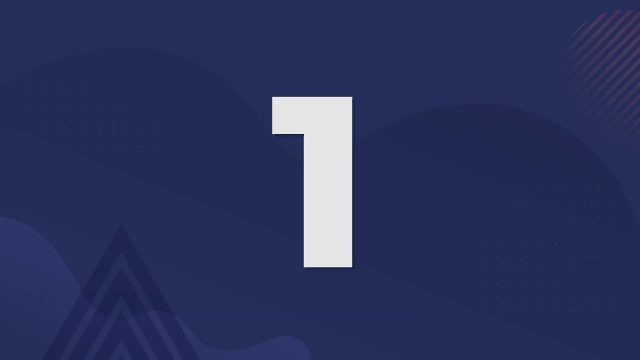 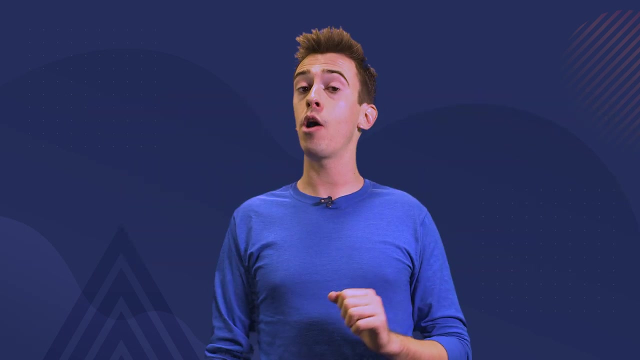 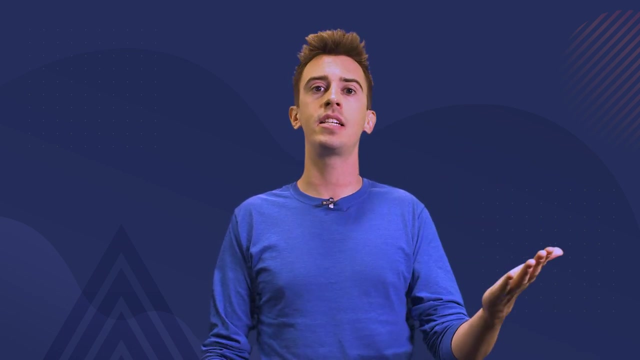 after they graduate. And the number one school on our list- no surprise to anyone- is the Massachusetts Institute of Technology. Now, MIT does not actually have a statistics department, but it is still the number one school on our list because they study statistics in many, many other departments. 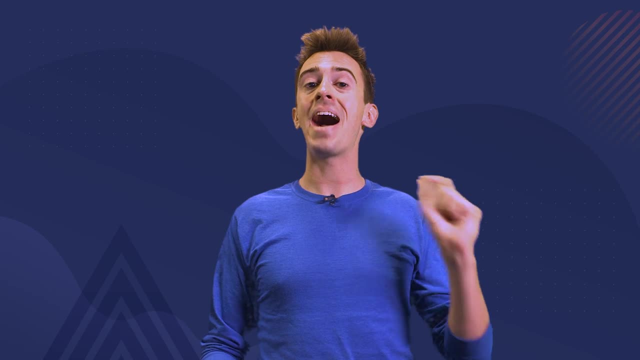 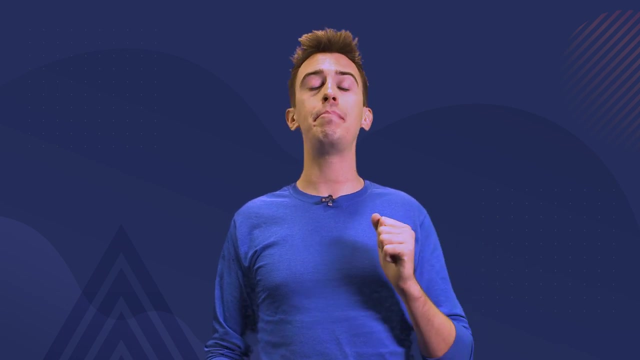 and they're the best in the world at doing it. You can, however, get a minor in statistics and data science at MIT, which is a pretty recent development, And after the undergraduate level, there is an interdisciplinary PhD in statistics that MIT offers, which much like its undergrad programs. 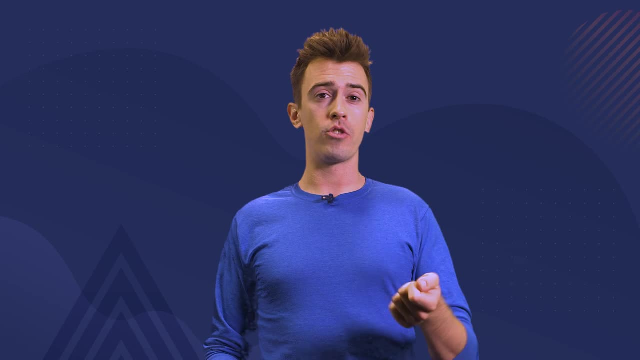 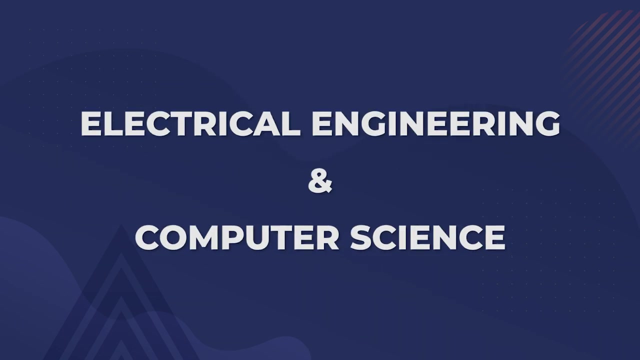 is the best in the world. MIT recommends that graduate students who are interested in statistics go to one of two research centers: The first is the Operations Research Center and the second is the Electrical Engineering and Computer Science program. So again, even though MIT does not strictly,